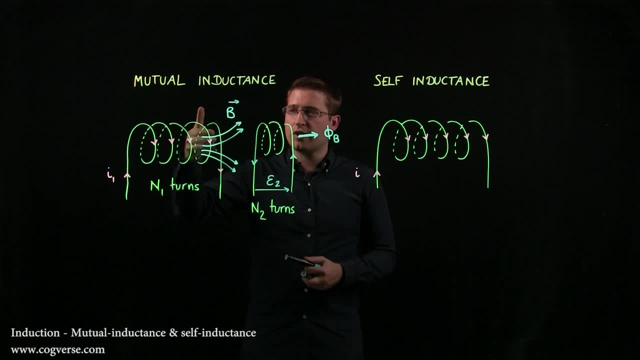 appeared because we changed I1, which changed the flux of b through this coil. So basically we increase I1, the magnitude of the flux, and then the magnitude of b goes up and the flux this way increases, creating an induced emf across the second coil. So the second coil is made aware of the first by 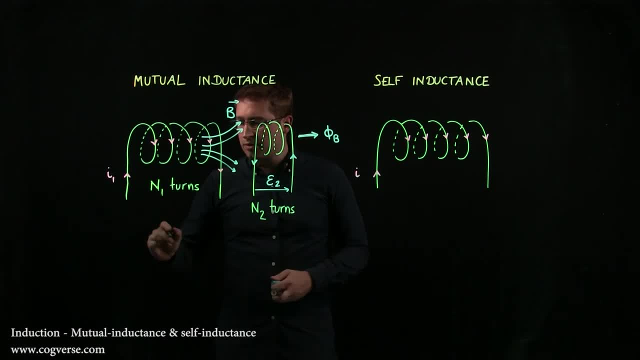 changing the current in it. and in fact epsilon 2 from Faraday's law, we know, is going to be proportional to dphi b over dt, but phi b itself is proportional to I1, and what we are going to write is that it's. 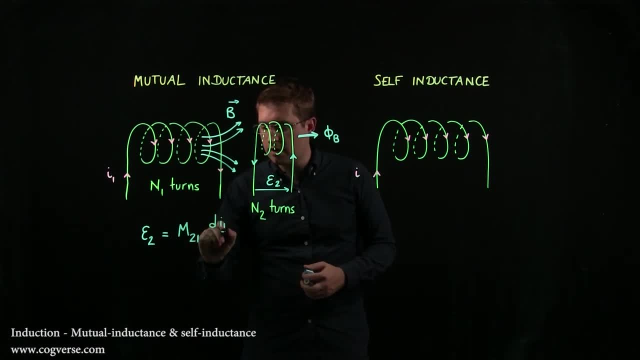 m21, d, I1 over dt and m21 is a constant coefficient and it's actually called the mutual inductance, and the mutual inductance has a unit that's called the Henry, but we'll get to that in just a second. So this is epsilon 2, and it is generated because of the change. 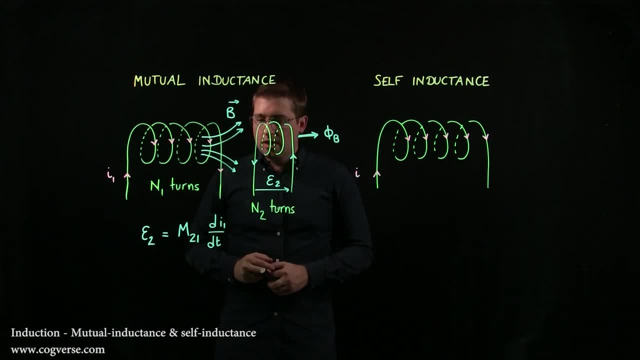 in I1, we ramped up I1.. Now you could argue: well, wait a minute, I could not do the opposite. could I not just run I2 through this one, increase it and then make the first coil aware of the second with the same kind of experiment? 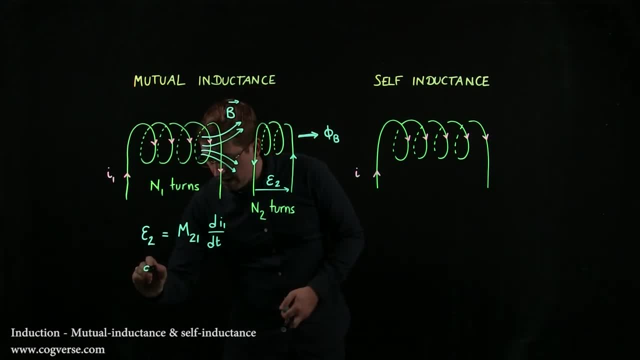 And yeah, sure you could. and you could also write, if you do that, that epsilon 1, the induced emf you'd get across this coil- would be m12, d, I2 over dt and that would be a coefficient called the mutual inductance. and the truth is m12 and m21 are equal, so we'll just use. 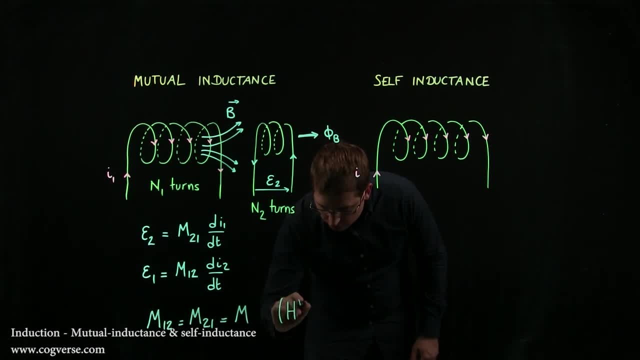 m, and the unit is Henry, which is denoted by uppercase H. So this is the mutual inductance coefficient, and we use it when one coil has an effect on another either this way or that way. Now, that's mutual inductance. Let's look at self-inductance, because the truth is: